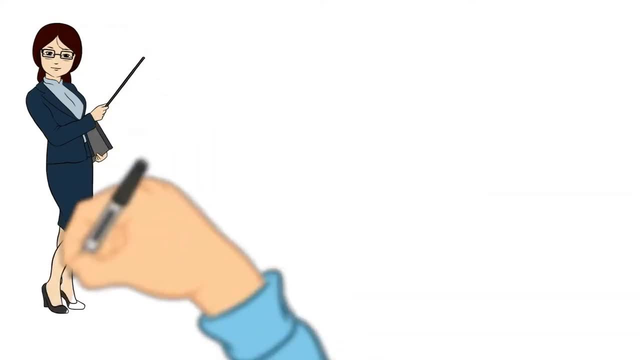 Our lesson for today is about addition. Let us start our discussion with the question. What is the definition of addition? 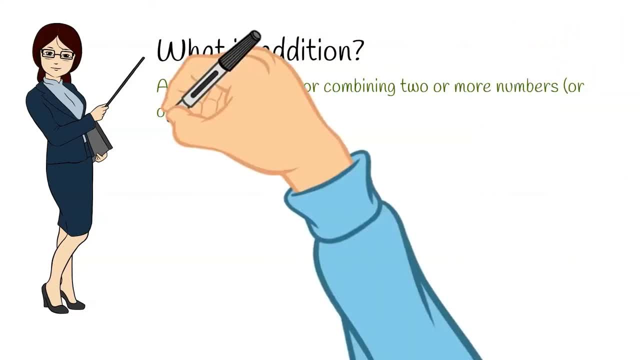 Addition is bringing or combining two or more numbers, or objects, together to make a new total. 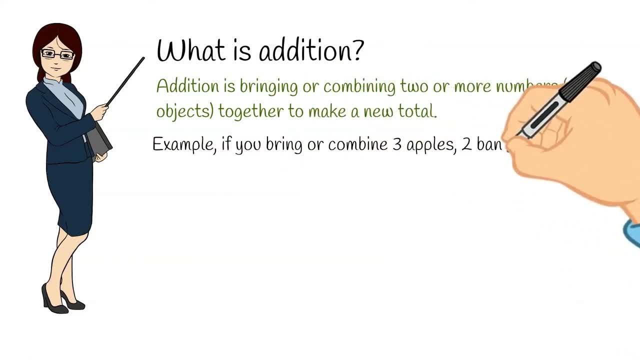 Example. If you bring or combine, three apples, two bananas and an orange together, you would have six fruits. 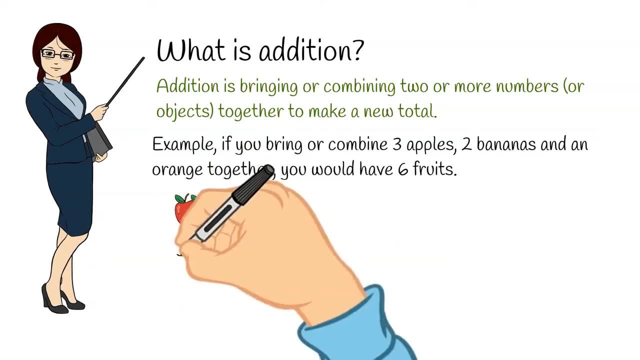 In this example, the given are. Three apples. 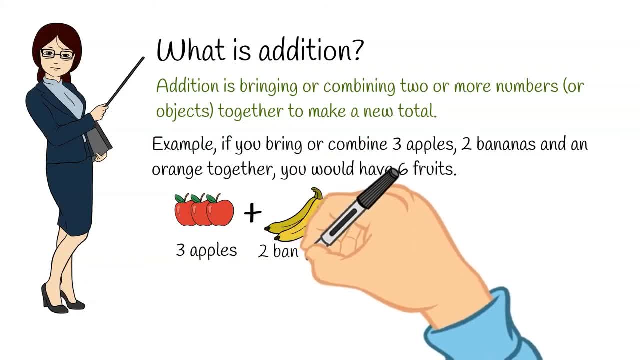 Two bananas. And one orange. If you add all these fruits, you will have. Three apples. Plus. Two bananas. Plus. One orange. Equals. 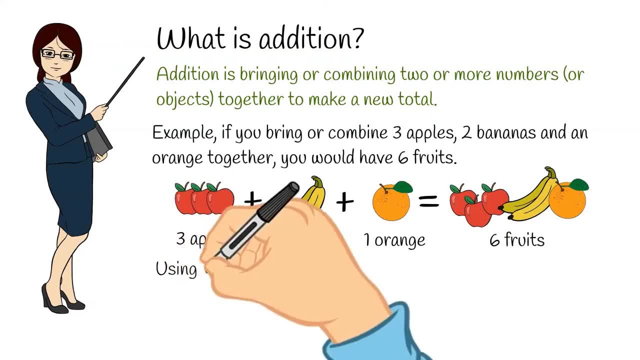 Six fruits. If you write this using numerals, it is. 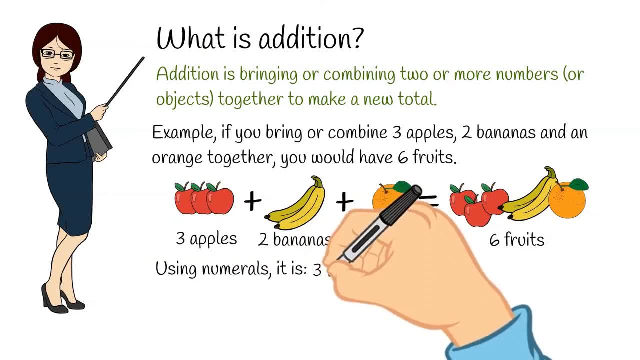 Three. Plus. Two. Plus. One. Equals. Six. 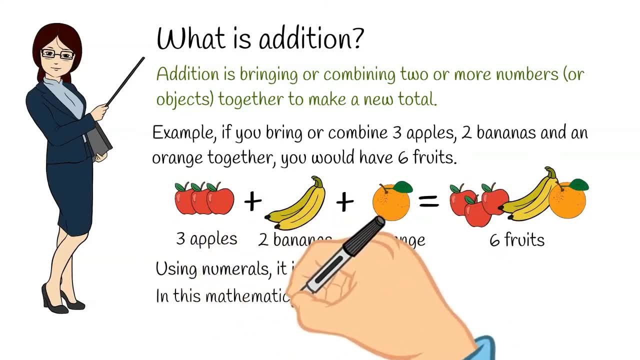 In this mathematical expression, the numbers three, two, and one, are called addends, and the number six, is the sum. 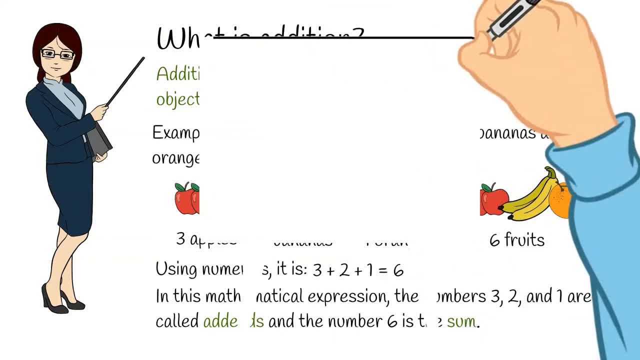 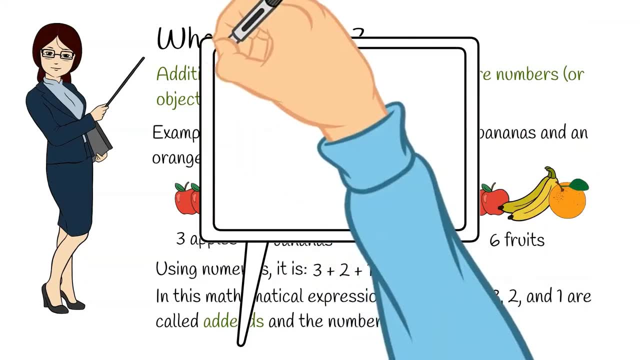 Perhaps one of the most common everyday uses for addition is when working with money. For example, adding up bills, receipts, daily expenses or savings. It is very important to learn the process of addition as this will help you all through your life. 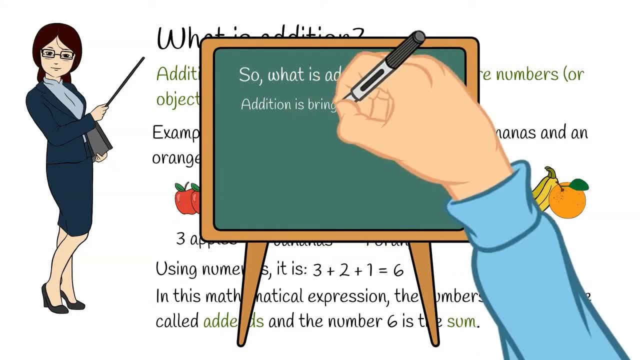 So, what is addition again? Addition is bringing or combining two or more numbers, or objects, together to make a new total. 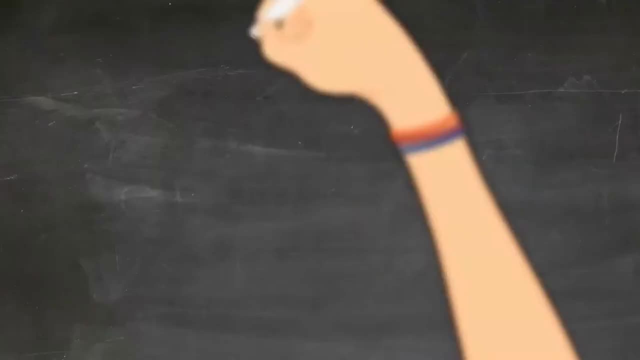 Let us have more examples. Welcome to Hippo Campus Learning Videos. 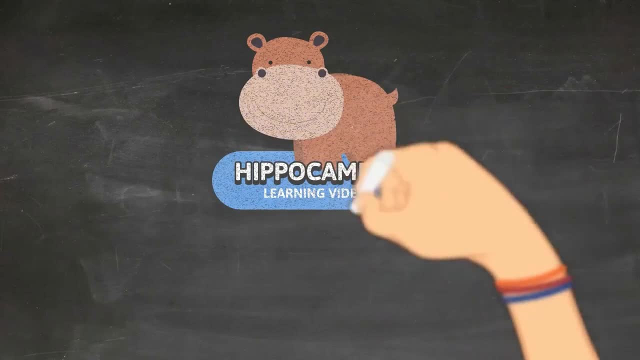 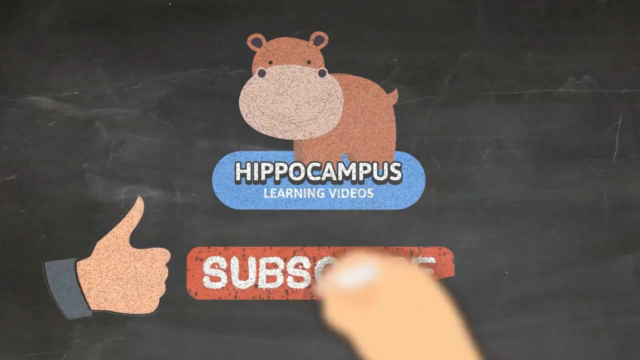 If you are enjoying the Hippo Campus Learning Videos, please give us a like, subscribe, and hit that notification bell so you can be notified when new learning videos are added to the channel. Happy Learning! 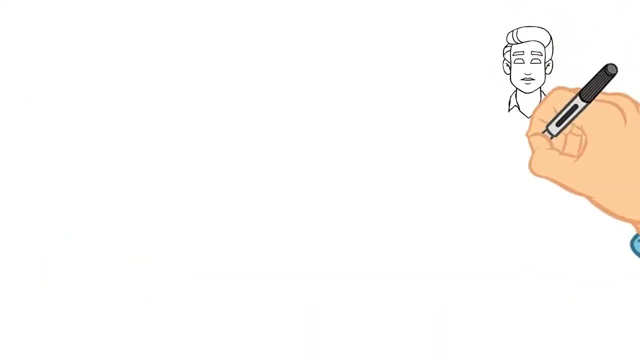 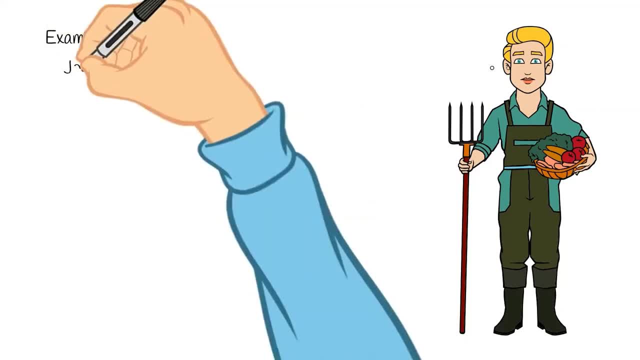 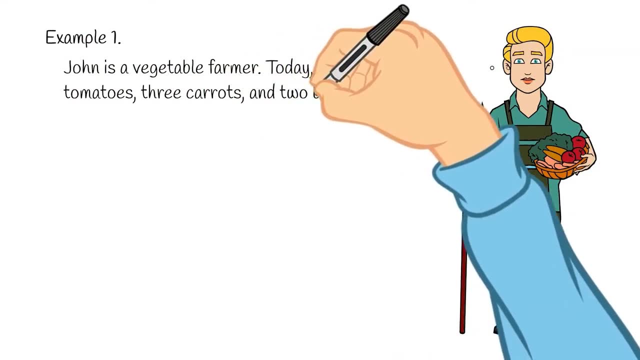 Let us use this scenario as example number one. John is a vegetable farmer. Today, he harvested four tomatoes, three carrots, and two broccoli. How many vegetables, in total, did John harvest today? 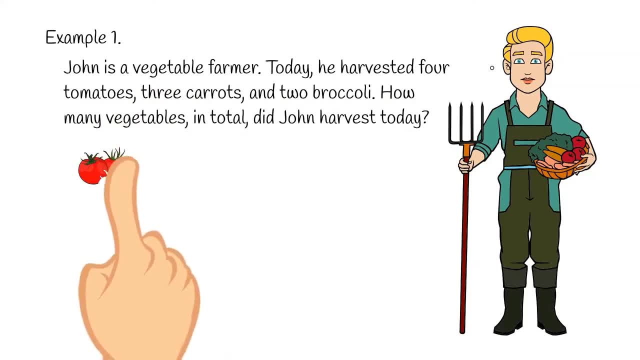 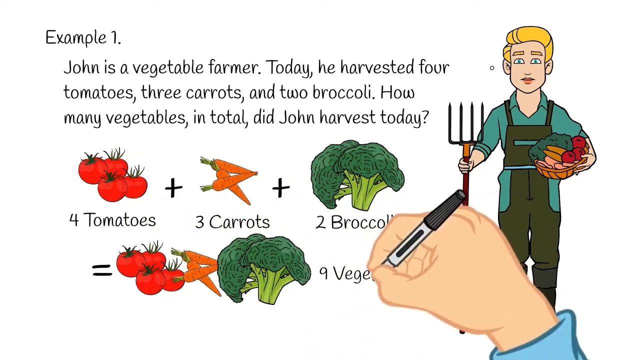 In this example, the given are, 4, tomatoes, 3 carrots, and 2 broccoli. If we combine all these vegetables together, the total number of vegetables will be, 4, tomatoes, plus, 3 carrots, plus, 2 broccoli, equals, 9 vegetables. 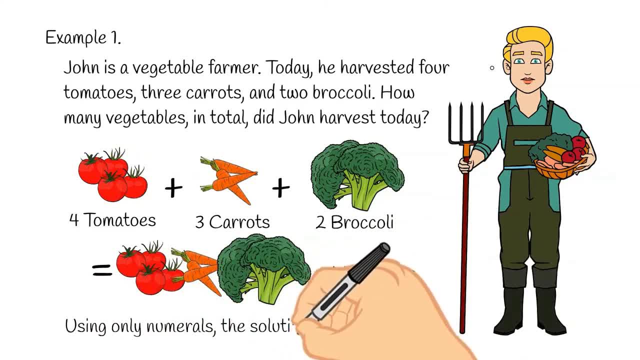 Using only numerals, the solution will be, 4, plus, 3, plus, 2, equals, 9. 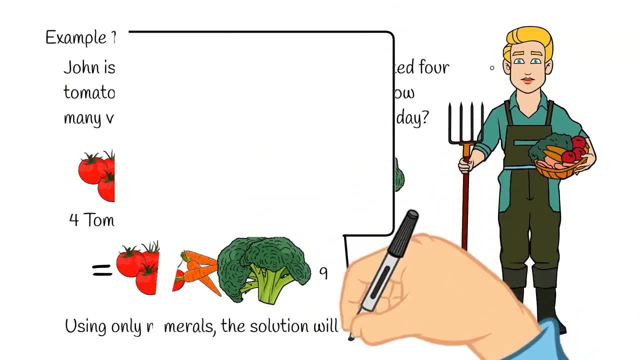 I am sure you are now starting to understand the importance of addition. 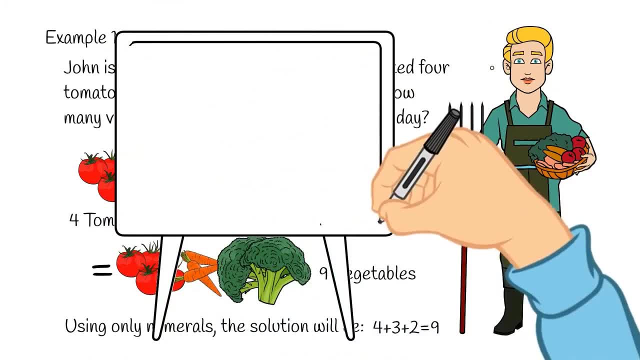 You can almost use it in everything you do, every day. Isn't addition fun? Let us go back to example number 1. Again, the solution is, 4, plus, 3, plus, 2, equals, 9. John harvested 9 vegetables today. 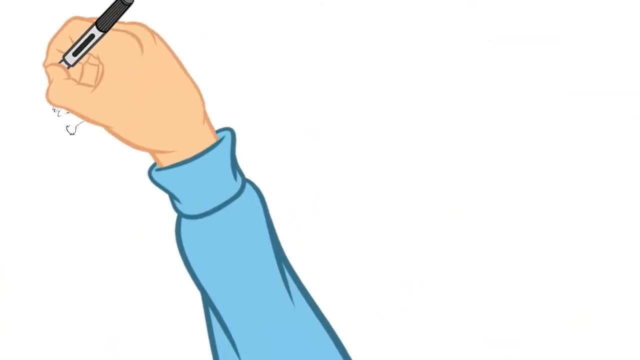 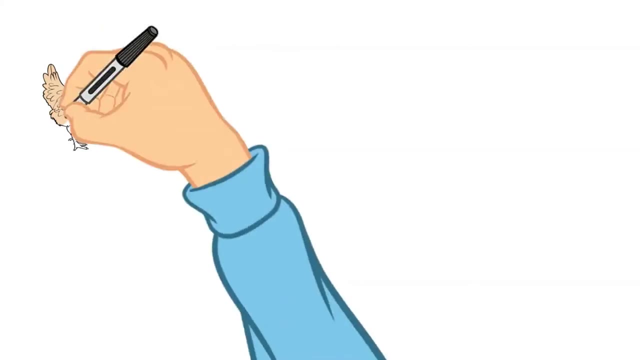 Addition can also be used in managing a poultry business. Using addition, you can calculate how productive your chickens in laying those delicious eggs. Let us have another example. Example number 2. 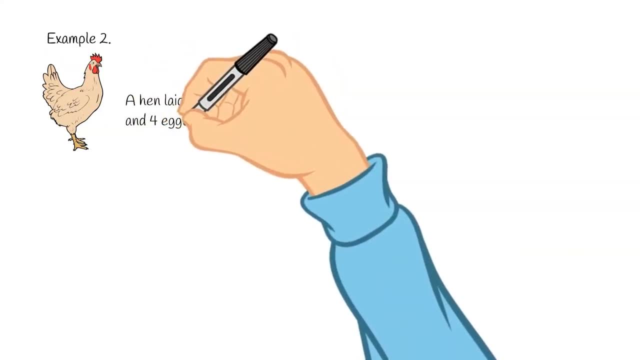 A hen laid 2 eggs yesterday and 4 eggs today. If it lays 2 eggs tomorrow, how many eggs will the hen have laid by tomorrow? 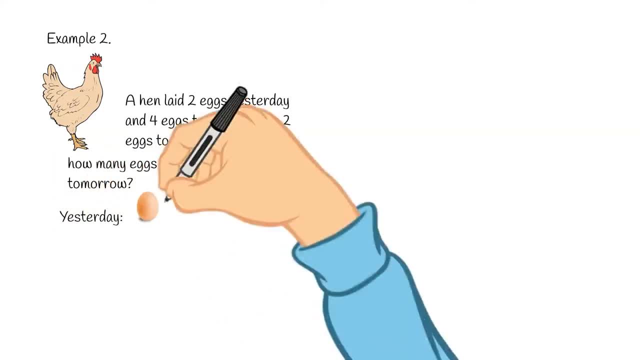 In this example, the given are, 2 eggs are laid yesterday. Today is very productive as 4 eggs are laid today. 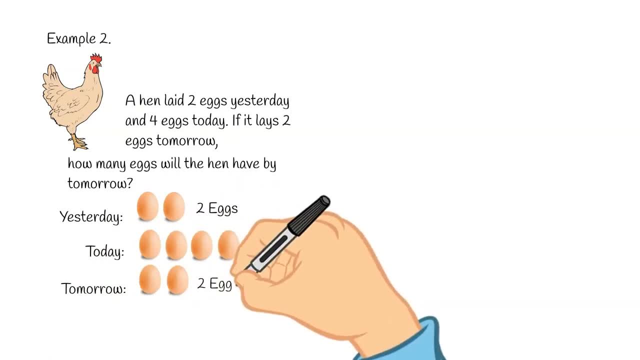 And 2 eggs are expected tomorrow. The solution is, therefore, 2. 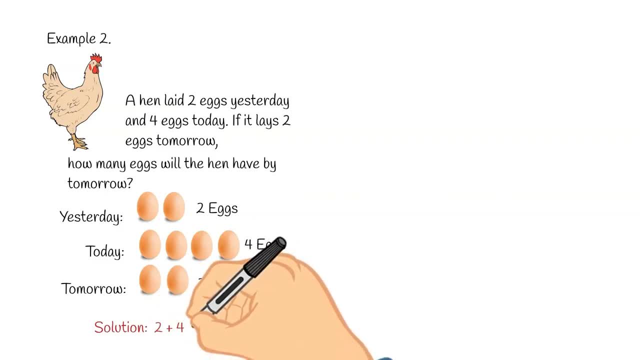 Plus, 4. Plus, 2. Equals, 8. 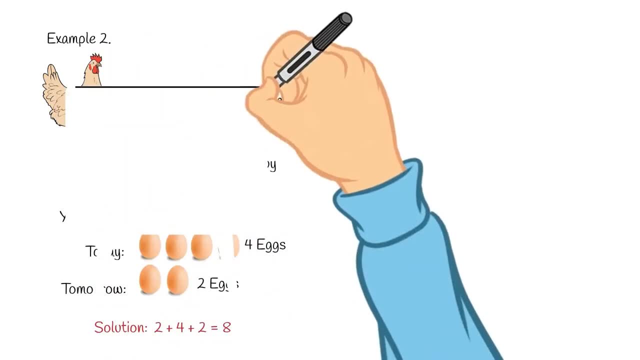 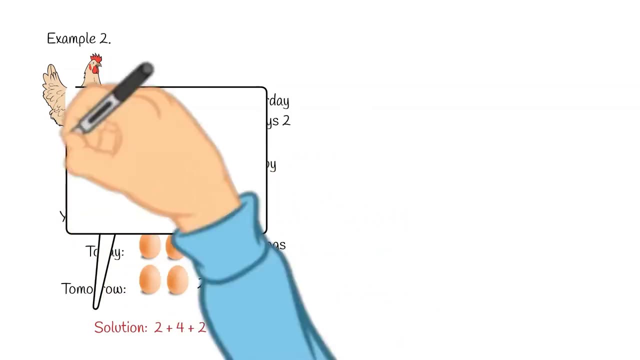 Addition cannot only be used in managing the productivity of a business. It can also be used in managing sales. In the previous example, addition can also be used in calculating how many eggs the poultry business is selling, making addition a very useful tool in making a living. 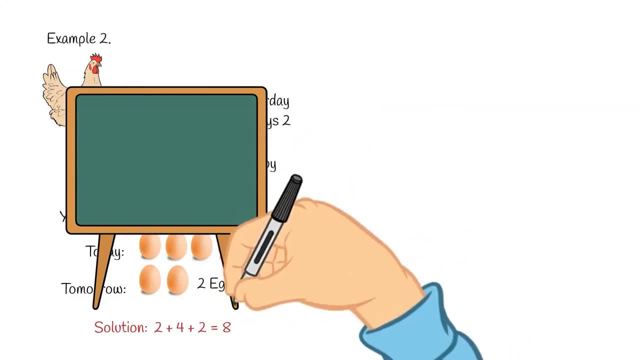 Going back to example number 3. Using addition again, again, the solution is, 2. Plus, 4. 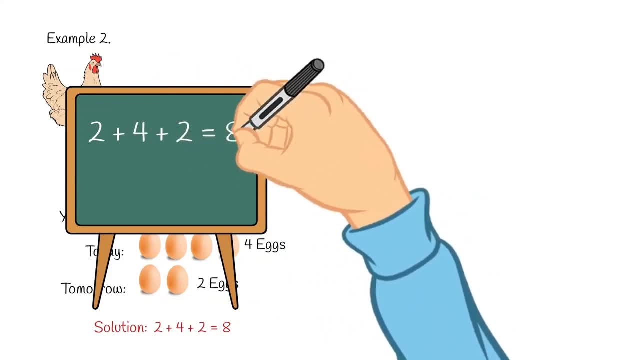 Plus, 2. Equals, 8. 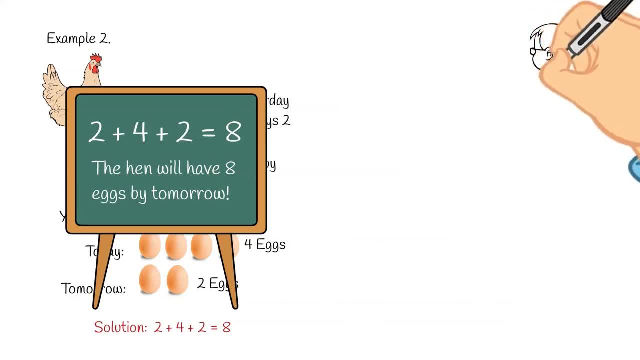 Another important use of addition, is managing our time. To be productive, we should be able to allot time to our daily activities, like doing household chores, work, rest, ты, outdoor activities, studies. Doing that would enable us to manage our time more efficiently, giving us more balance in life. Let us have one more example. Example number three. 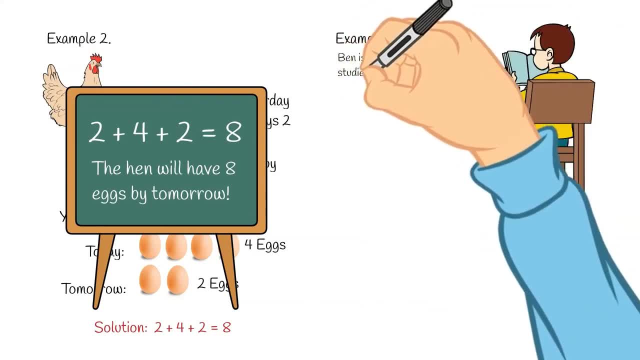 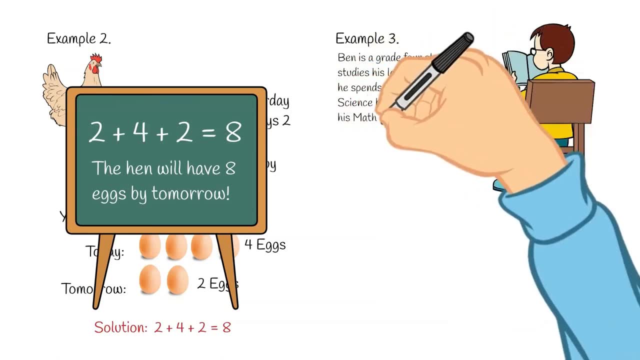 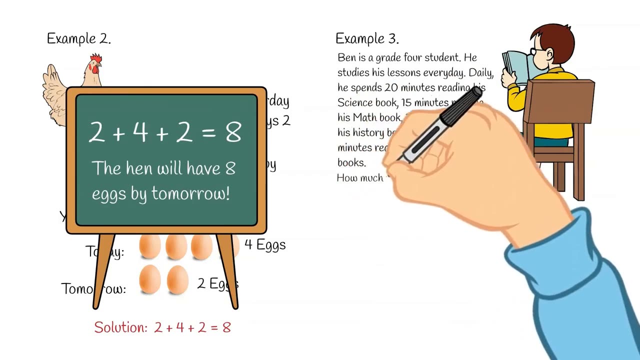 Ben is a grade four student. He studies his lessons every day. Daily, he spends 20 minutes reading his science book, 15 minutes reading his math book, 10 minutes reading his history book, and another 40 minutes reading the rest of his books. How much time does Ben spend reading every day? In this example, the time Ben spends reading his book on a daily basis is being asked. 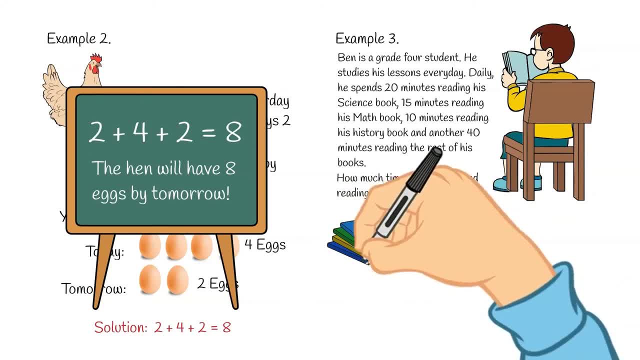 So, what are the given information? Ben spends 20 minutes reading his science book, 15 minutes reading his math book, 10 minutes reading his history book, and 40 minutes reading his science book. 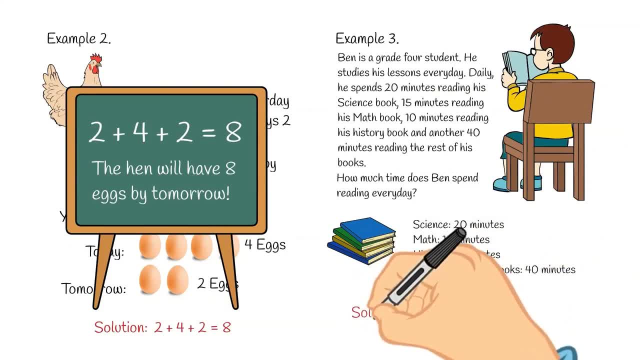 40 minutes reading the rest of his books. The solution therefore is 20 plus 15 plus 10 plus 40 equals 85. Addition has infinite number of uses. We use it every day and always. 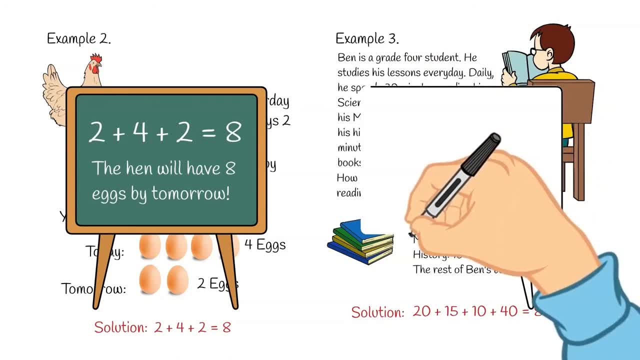 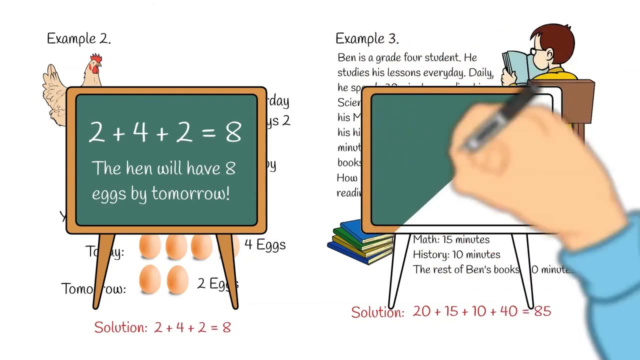 When you count your things, you use addition. When you manage your time, you use addition. When you want to be productive, you use addition. When you are saving for the future, you use addition. Now, I am sure you are realizing how often you use addition and how 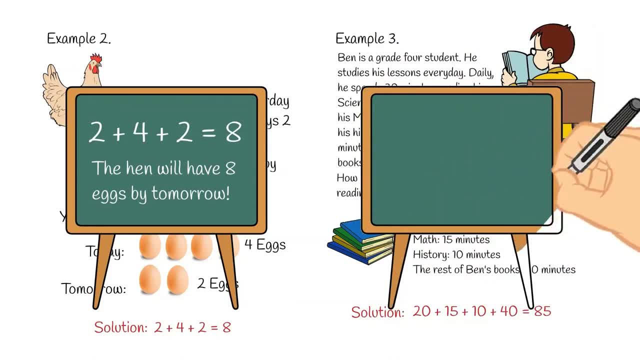 important it is to you. Let us go back to example number three. Again, the solution is 20 plus 15 plus 10 plus 40. 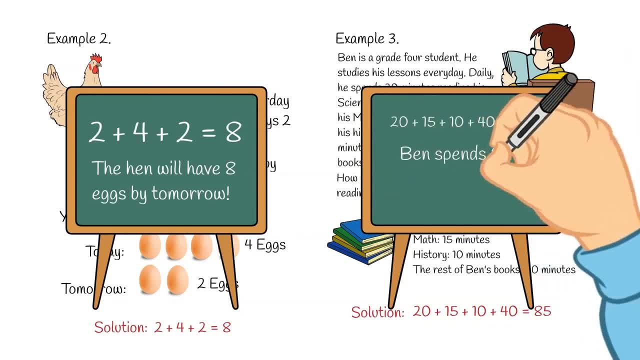 Equals 85. Ben spends 85 minutes reading his books daily. 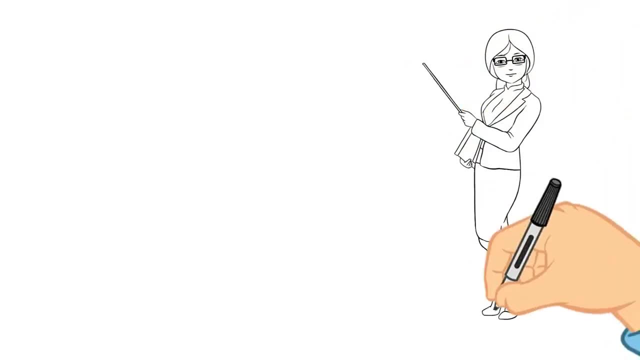 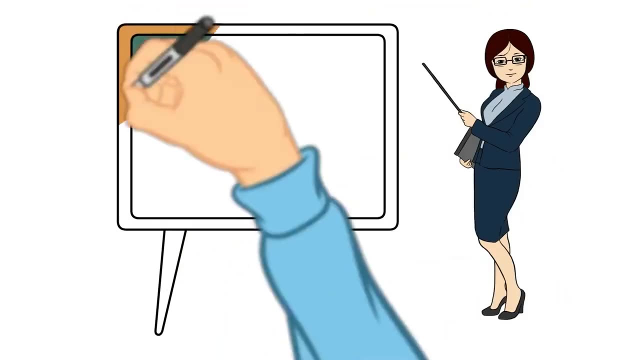 We have come to the end of our topic at this time. I am sure you now understand and realize the importance of addition in our daily lives. But before we end, let us revisit the definition of 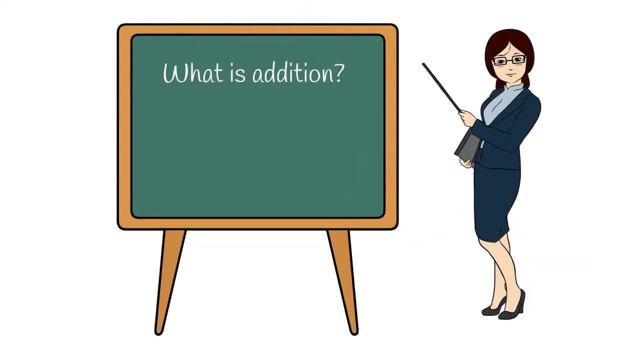 addition again. What is addition? Addition is bringing or combining two or more numbers or objects together to make a new total. 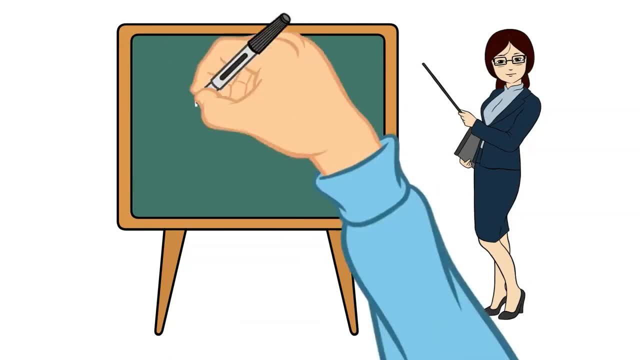 Thank you for studying. Happy learning. 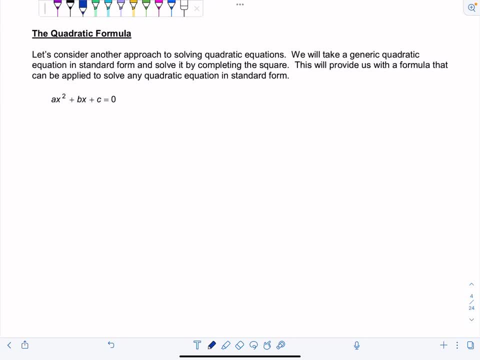 Welcome to Mac TV with Professor V. In this video we're going to learn about the quadratic formula. This is part of the intermediate algebra video lecture series and if you'll recall in the previous lesson we went over how to solve quadratic equations using the square root method as well as by completing the square. And now we're going to learn another method which is using the quadratic formula. So the quadratic formula actually didn't just pop out of thin air. It comes from completing the square on a generic quadratic equation that's written in standard form. So remember quadratic equations occur when the highest power or exponent on the variable is a 2 and in standard form we have them written with all the terms on the left in descending powers set equal to 0 like this AX squared plus BX plus C equals 0. So say I wanted to go ahead and solve for X in this equation by completing the square like we did in the last lesson. So what would you do? Well first things first I'd move that constant C to the other side. 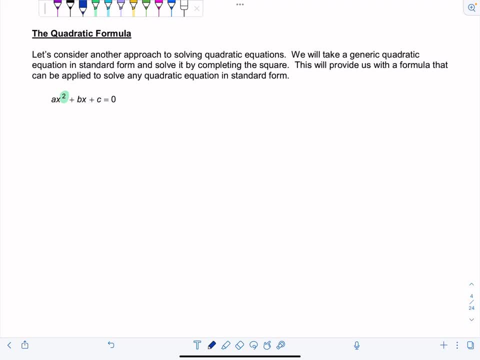 So here we would have AX squared plus BX equals negative C and then remember we're going to use the quadratic formula to solve this equation. 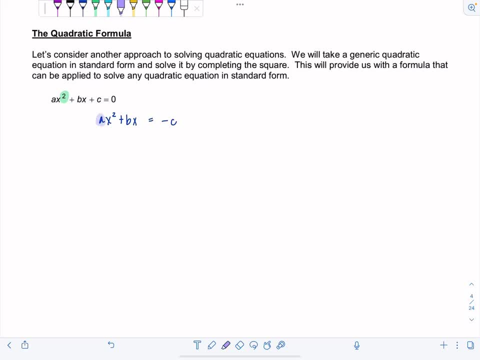 And remember we only complete the square when the coefficient on X squared is a 1. So if it's not a 1 we divide through by whatever it is so I'm going to do that right now. And for the sake of this discussion right now, we're just going to assume that A is positive. That A is greater than 0. So now I have X squared plus B over AX X squared plus B over AX plus CARTERA. 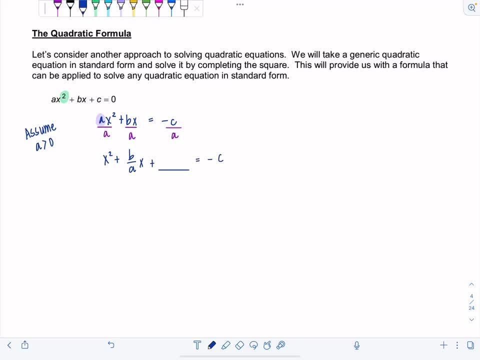 Plus, I'm going to try to figure out what I need to add to complete the square equals negative C over A. And remember, I'm going to add the same thing over there as well.